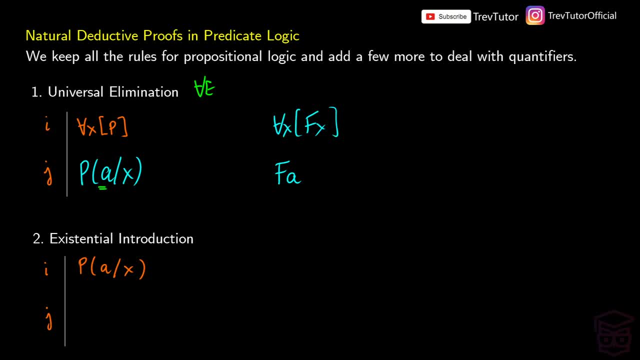 So this is universal elimination, This is for all, with an e beside it. So if you watch the truth trees, it's very similar. Existential introduction works sort of the same way. So imagine we know for a fact that we have, Let's say, p, c in our proof. 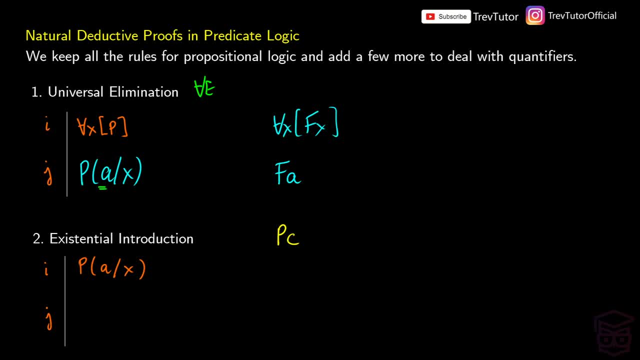 What we can do, then is, because we have at least one thing with the property c, we can introduce an existential and say there exists an x such that p x, Because all this requires is that at least one thing has the property p. We already assume something has the property of p. 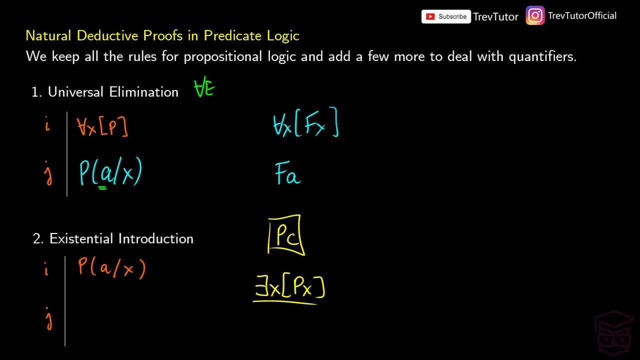 So we can say: okay, at least one thing has it. So if we have a formula where all of the x's have been replaced with something a, we can then say there exists an x, such that p. So just introducing that existential. 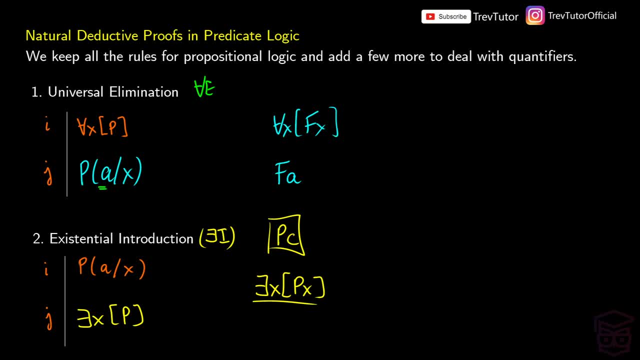 And this is a backwards e with the i for existential introduction. So these ones are straightforward. We don't have to worry about any sort of weird requirements on our constant a. But when we think about universal introduction and existential elimination we have to think about some extra requirements. 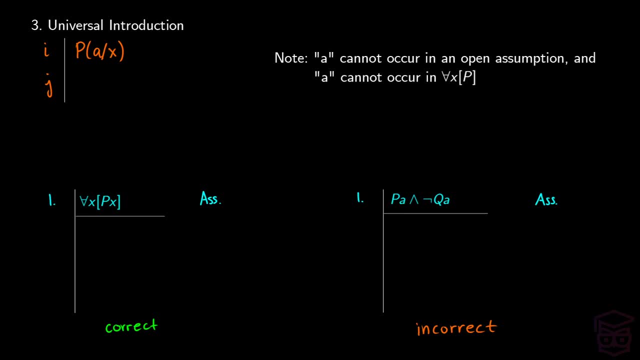 So let's take a look at each, Let's think of those rules. Okay, If we want to introduce the universal, it looks very similar to existential introduction. We have some formula p where we have a bunch of a's in there and they've been replaced with whatever x is. 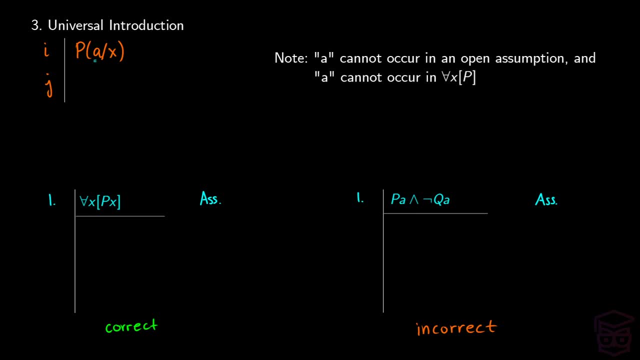 So in other words, we don't have an x in there, We just have some constant. Then we could say for all x, p. But there are two requirements about our constant here. If we want to introduce the universal, we have to have some constant. So if we want to introduce the universal, we have to have some constant. If we want to introduce the universal, we have to have some constant. So if we want to introduce the universal, we have to have some constant. So if we want to introduce the universal, we have to have some constant. 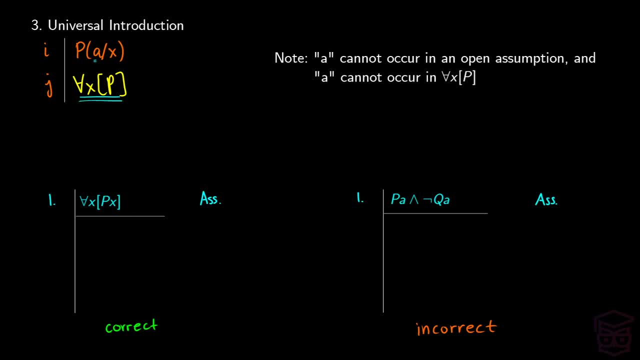 First of all, we cannot still have a's in this. We have to replace all of the a's. And second, the a's that we're replacing cannot have been introduced in an assumption, Because we're assuming something exists, So we can't claim that everything has that property. 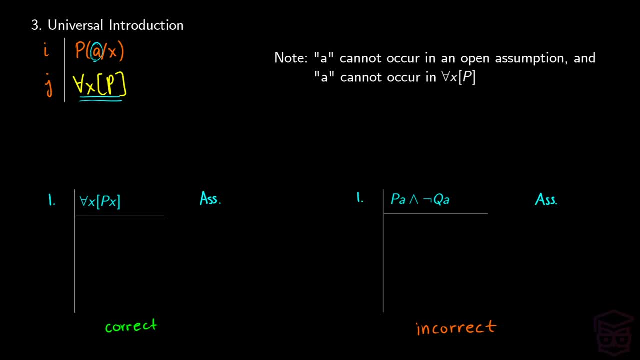 So these are the two things we have to look at, And I want to show you an example of using this correctly and an example of using this incorrectly. incorrectly, so that way we can wrap our minds around it. so imagine we start with for all x px. 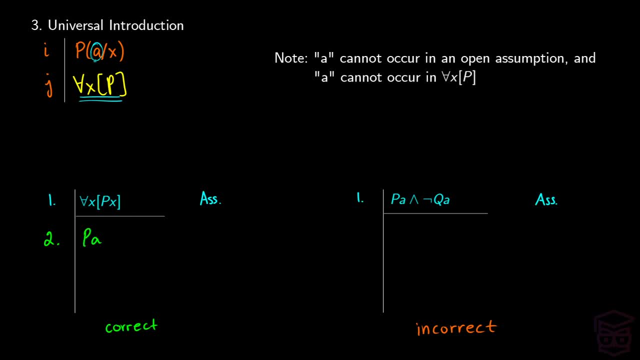 and from this we say, okay, we have pa and we can do this from x, from universal elimination, okay. now what we can do is we can say: for all, y, py. we can make this claim because, first of all, a does not appear in line three and the a that we had in two that we used to get. 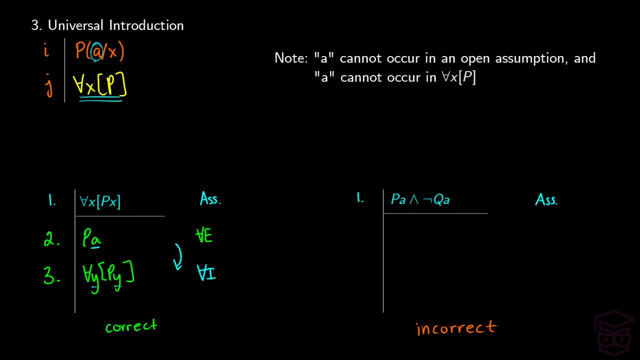 our universal introduction, so we can call this for all. i this a here is not in an assumption. this was a rule that we applied earlier. it doesn't appear in any of the assumptions, so we can do it. but if we take a look on the right side and see this working incorrectly, imagine: okay, we have pa. 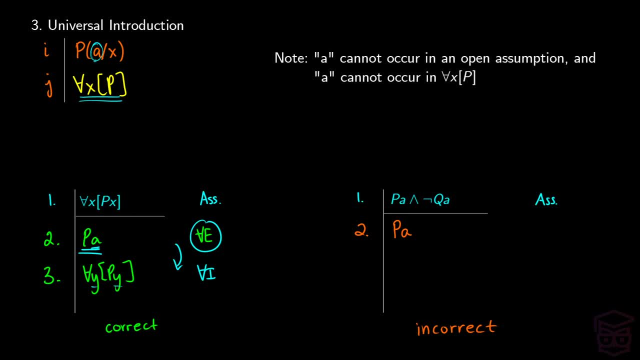 and not qa. we have a and not qa, and we have a and not qa. so we take pa it's line two. this is and elimination. now, what we cannot do in this case is we cannot say for all x px. so this one is wrong. and it's wrong not because a doesn't. 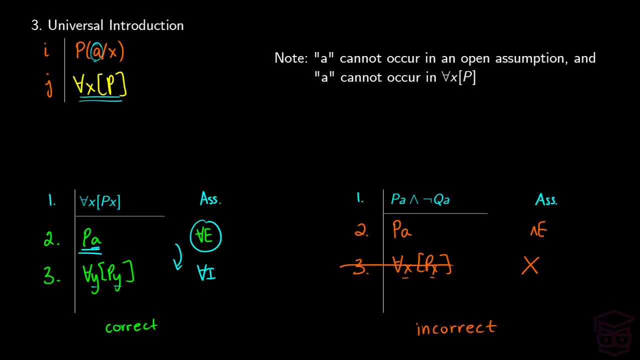 appear in there. that's fine, but the fact is that this a came from an assumption, so we cannot introduce the universal when we're working with a constant that has. that came from an assumption. uh, compared to this first one where, yeah, we still had an assumption about for all x px, not about a specific constant. so we'll see this in action again when we 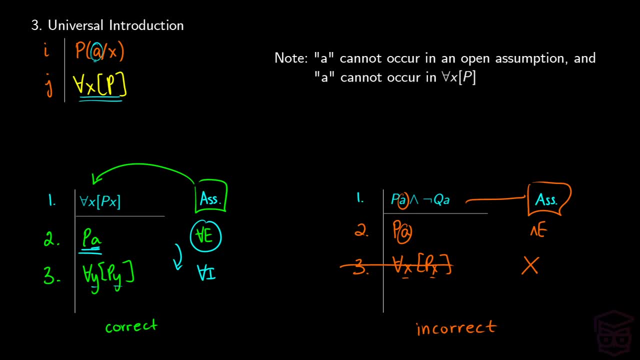 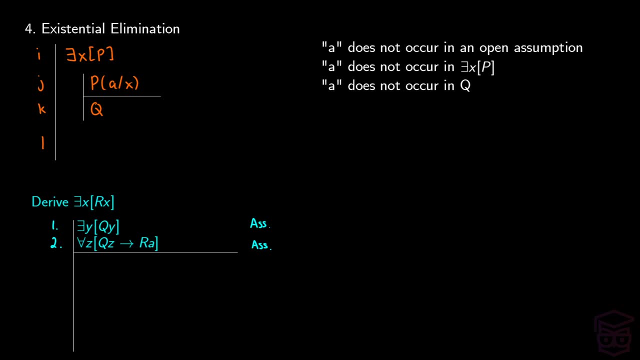 do the practice proofs. but i do want to introduce one more rule to you, which has very similar constrictions, so existential elimination, and this one is one of the more complicated ones. so let's just walk through the intuition of this. suppose i tell you that there exists an x such that px. 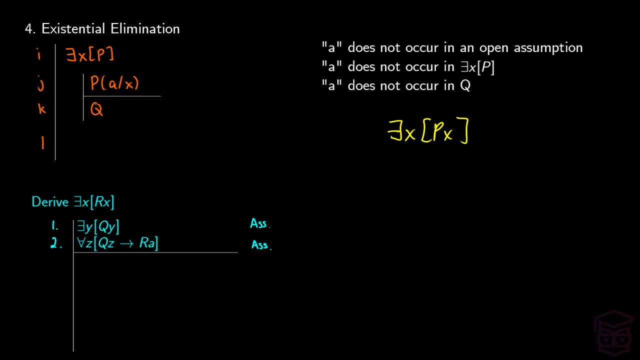 okay. so what i need to do in this case? if i know something has the property of p, i don't really know what it is, but i can say: okay, hypothetically, what if a has the property of being p? so i have this little sub proof here and i might derive something and i might find: oh, if a has the property of b. 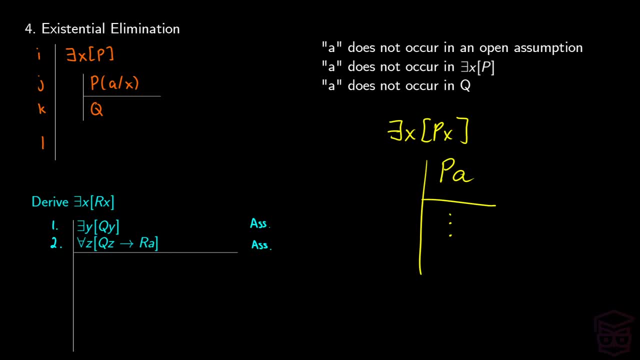 and p. then something else happens. let's say: then b has the property of being q. so as long as our final result here is not a, so in other words that assumption is still not in that assumption, as long as a doesn't occur in the original thing- uh, then we can claim: okay, no matter what thing we assume has the 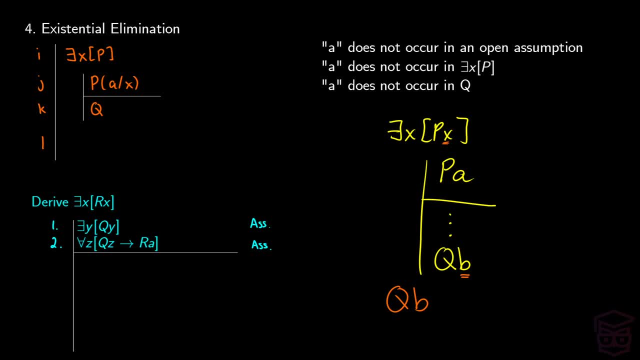 property of being p, we can get qb out of it. so this is our hypothetical. we ask ourselves: what do we get with that hypothetical? and as long as whatever we get doesn't involve our assumption about a, we're good. so in terms of on the left side, the formal proof there exists an xp, we assume something where a. 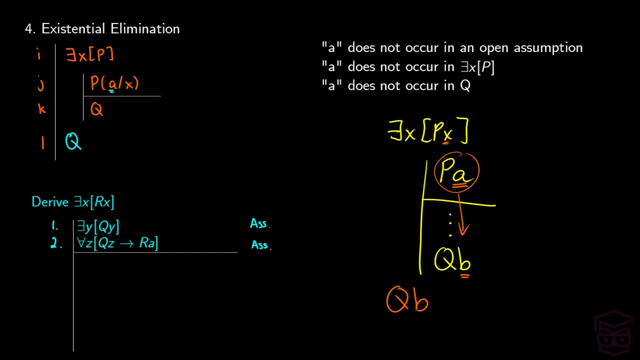 replaces x, we get q out of it. then we can claim: okay, we got q from that. so let's see this in action and hopefully that makes a little bit more sense when we see it working. so three we have: exists: a, y, q, y and for all, z. if qz, then ra. so let's ask ourselves, let's introduce: 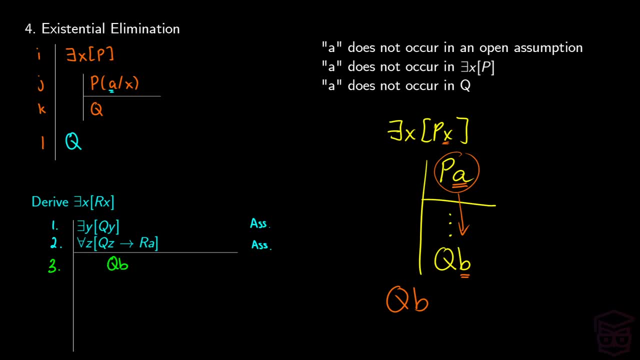 a new variable and say what happens if we assume that some variable b has the property of being q, so this is qb, and sure we'll introduce a little line here to make it nice and we'll call this an assumption. so what happens? well, in line two i have universal z. 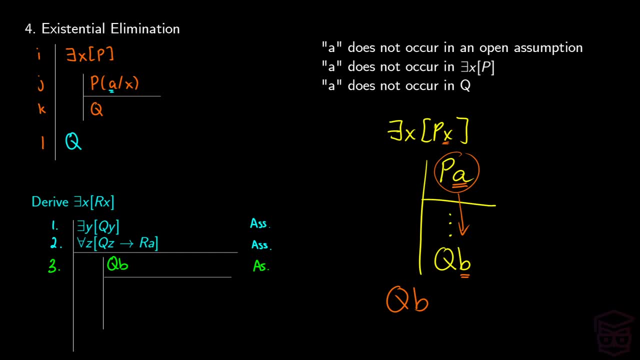 z arrow ra, so i can replace z with whatever i want, with universal elimination. so i can say: okay, if qb, then we get ra. so this is from two, this is universal elimination. now, from three and four we have qb. if qb we get ra, therefore we get ra. so from lines three and four we do modus ponens and 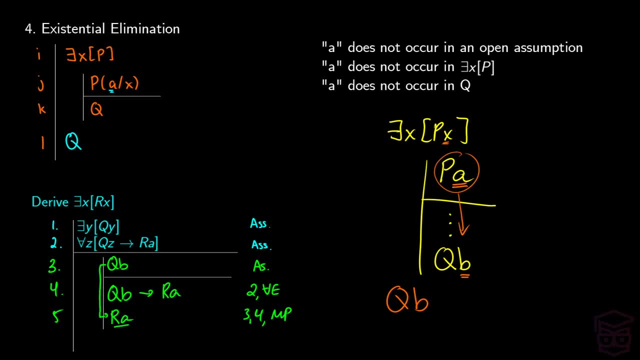 now qb to ra. we're looking at the constant. a does not occur in our assumption about exists a, y, q, y to qb and we also don't have this constant here. so b is different than a. therefore we can claim: in line six, from uh three to six, we did existential elimination, so no matter, uh, what thing we 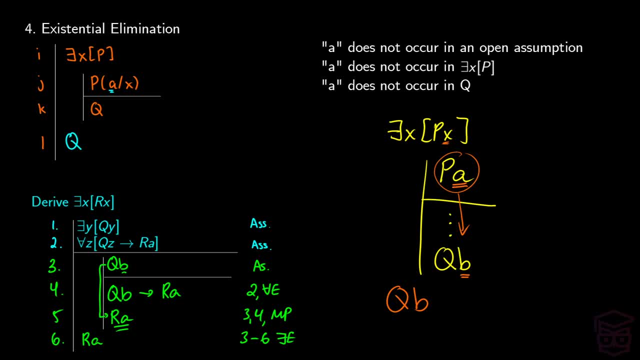 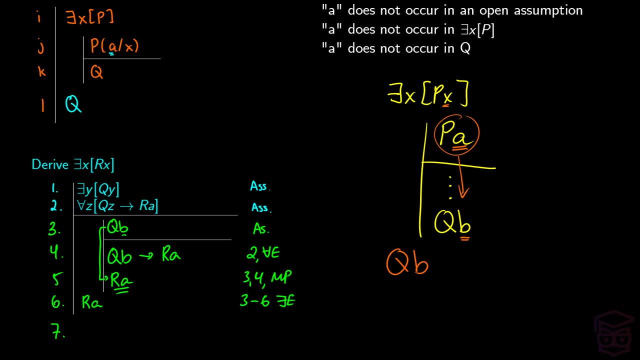 say, has the property of being q, we're going to get ra out of it. and now in line seven, so there's our experien Fraktion entry. so what we need to solve is so, when we ours r and then ánding a of r and r, because we have something that is r a. 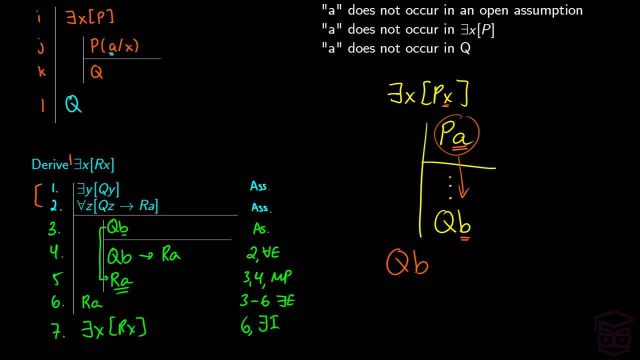 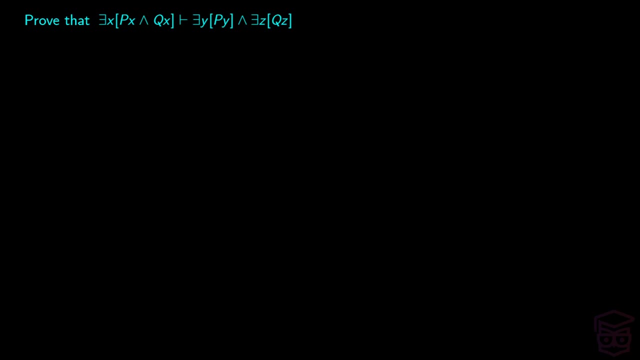 we can introduce the existential and say: okay, that means there exists an x such that rx. so from six we did existential introduction and now from our two assumptions here we have derived: there exists an x such that rx. okay. so now that we've shown the rules, let's 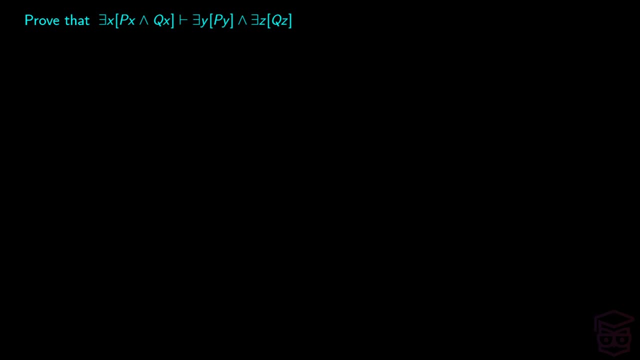 Let's do two more practice proofs: px and qx. then we find that there is some y that py, and there's some z that pz. So let's set up our first assumption. So let's assume there exists an x such that px and qx. 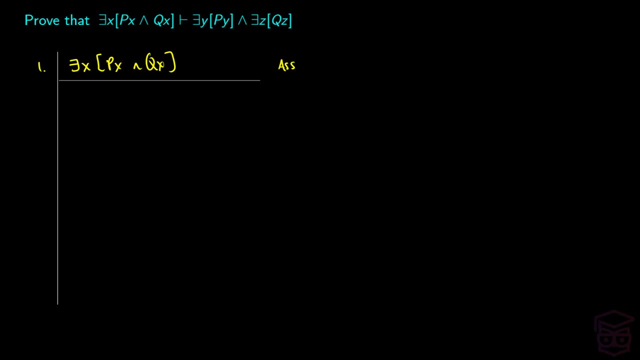 So let's call this an assumption, And this is all we have to go off of. So what we're going to do is we're going to assume: okay, there's something out there that is px and qx, let's call that a. 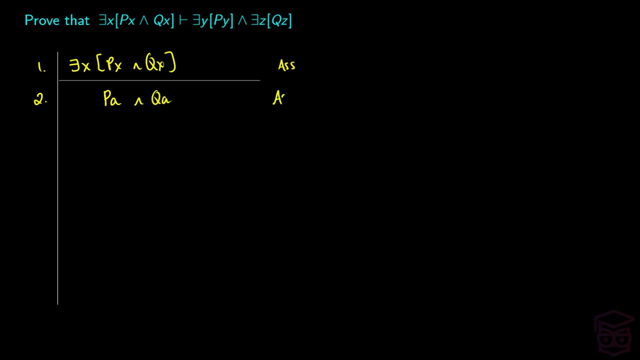 So I'm going to assume pa and qa for a subproof and let's see what we get out of it. Okay, well, two things: In 3, I know we have pa and in 4, I know we have qa. 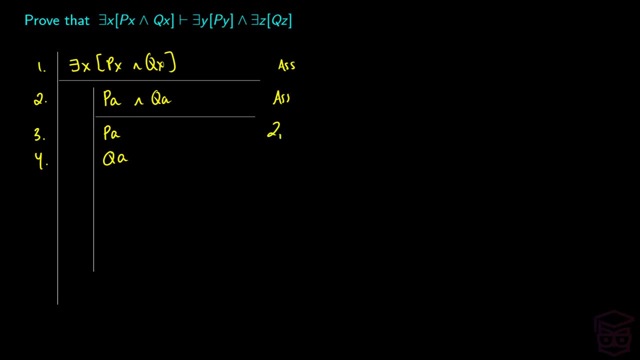 And we get this because we can do- and elimination on 2.. That should not be 3, that should be 2, right there. Okay, now, because we have pa, we can do existential introduction, And there's nothing wrong about doing existential introduction. 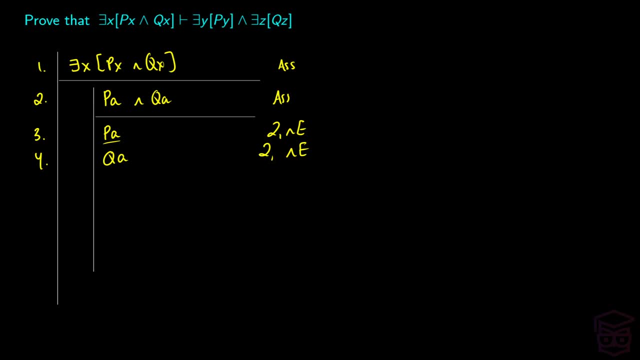 on some constant that's been in an assumption. We're not limited by existential introduction for that. So on 5, we do have to pick a new variable, though. So let's do exists a y, py, because that's what we want it to do. 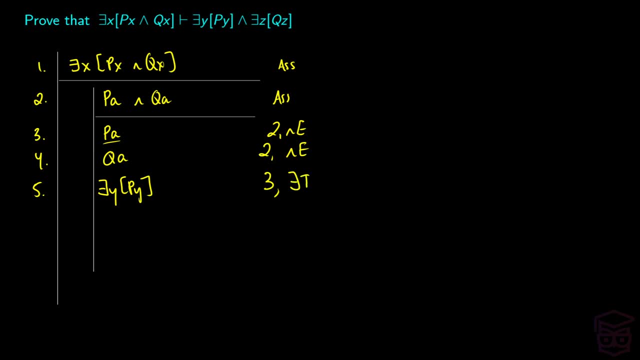 So this is on line 3, and this is existential introduction. Let's just do: exists a z, qz at the same time, why not? So on line 4, we have qa, so we can introduce a new variable and say there exists a z, such that qz. 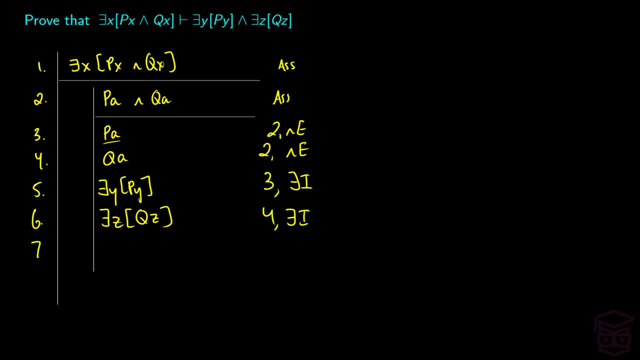 So from 4,, that's another existential introduction, And in 7, we can take 5 and 6, and we can compound them together. So exists a, y, py and exists a, z, qz. So from 5 and 6,, that's and introduction. 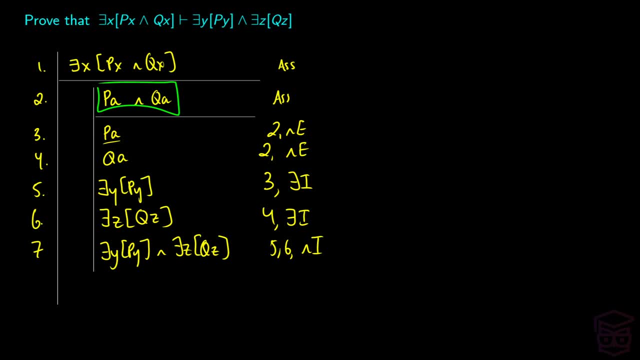 Okay. So now we've made an assumption, pa and qa. We've got a result. It doesn't contain any a's. It also doesn't contain the original exists and x there. So all of our requirements are satisfied. So now we can say that we get exists a, y, py and exists a z, qz. 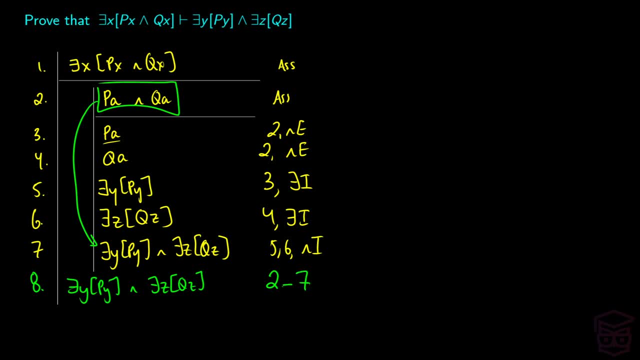 And this was from 2 to 7: existential elimination. So, based on our one assumption about saying, okay, this thing has the property of being p and q, we get there's something with the property p and something with the property q. 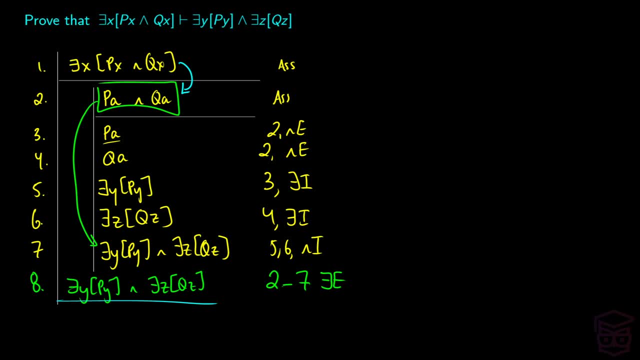 So that is our first proof. Now we didn't have to do both of these inside We could have done like one sub-proof where we got exists a, y, py, and then we could have done another sub-proof where we got exists a, z, qz. 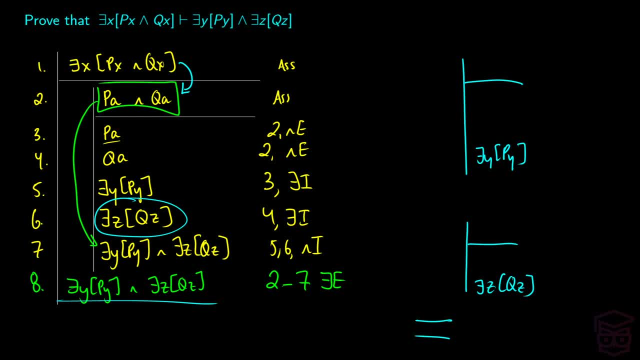 and then we could have compounded them together outside. That would have been fine. However, I just wanted to make sure that we were able to do that. I wanted to make the proof a little bit shorter, so I did them both at the same time. 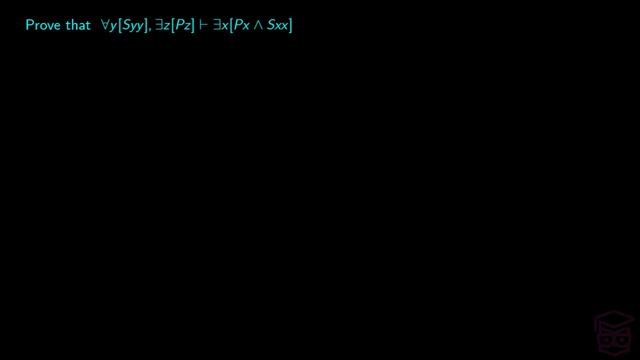 Okay, one more. Let's prove that for all y, syy, and there exists a z, such that pz, means that there exists an x, such that px and sxx. Okay, so, intuitively, basically, everything is syy, so everything in the universe. 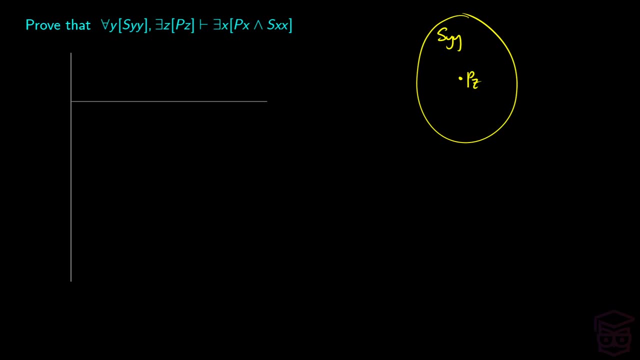 There's something here that is pz. There's something here that is pz. There's something here that is pz. Therefore, there's going to be something that is both sy and pz. That's essentially what we're saying here, And intuitively, we know this is true. 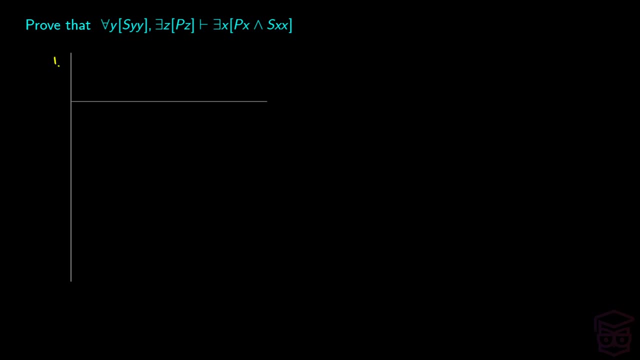 so we should be able to construct an argument for this. Okay, so for one, we're going to write down our premises. So this is for all y syy. There's an assumption, Two exists: a, z, such that pz. There's another assumption. 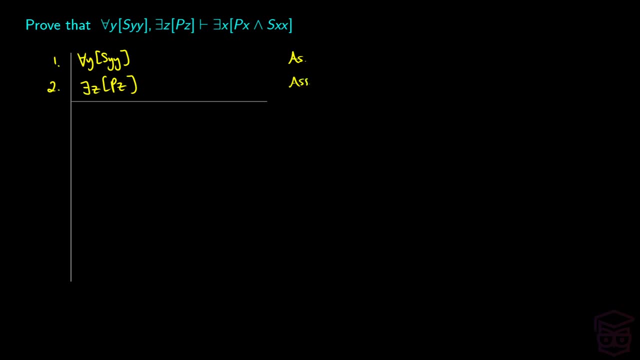 So what do we do? Well, let's start by assuming something for the x, and we're going to do an existential first and do a sub-proof. see what we get. So we know there's something that has the property of being p. 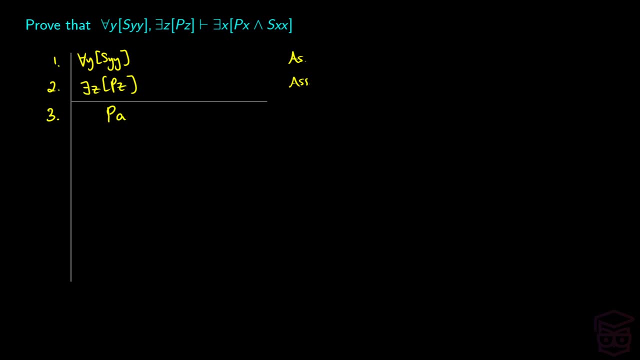 so let's pick p a, Why not? So we'll start a new sub-proof here. I don't know how long it's going to go, but this is another assumption. Now, what do we have here? There's nothing really we can do with the p a here. 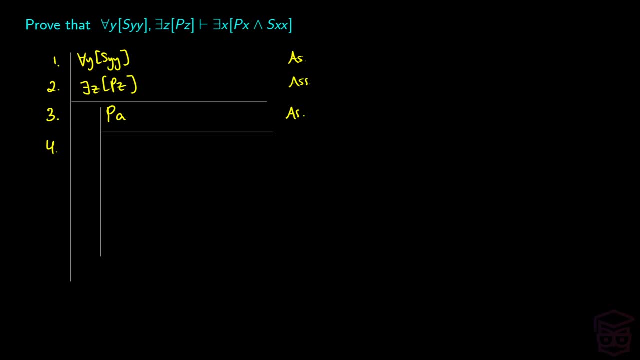 so let's use our universal rule. So we have s s a a because for all y, s, y, y, so we can use on one universal elimination to get s a a. Okay, we have p? a and s a a. 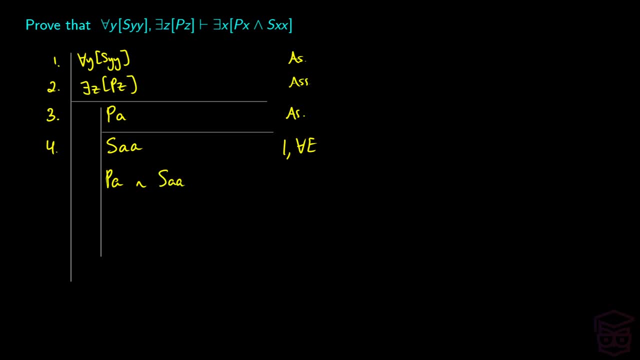 so I guess what we can do is we can join them together, p, a and s, a, a, So from three and four, that's conjunction introduction. And now what? Well, we do the same thing we've done before. 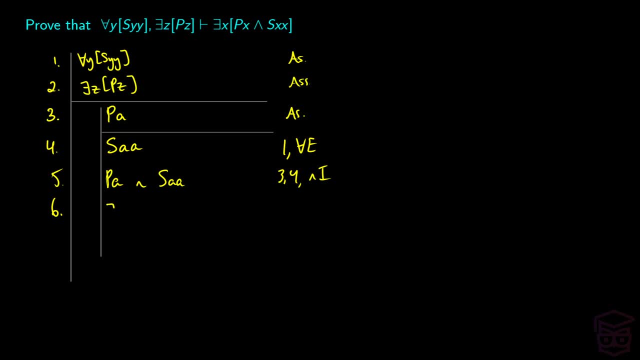 We know p a and s a a, So we can say that There's some x out there, that is, p x and s x x, because we have to replace all of the a's with x's. 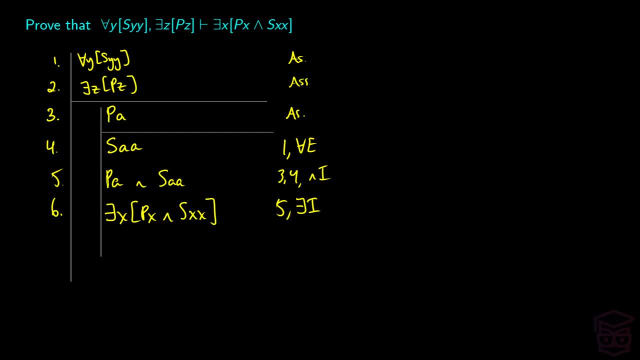 So from five, that's existential introduction. Now we assumed p, a. We've got something that has no a's in it at all. Therefore, with existential elimination we can remove this final thing that we've got. So it exists in x, p, x and s x x. from six: 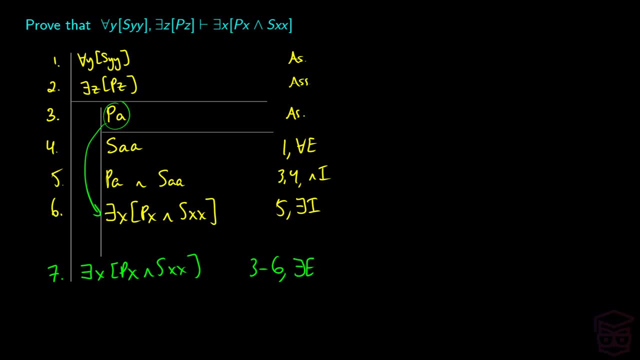 Sorry, This is from three to six. We have done existential elimination And we've proven there is some x, that's that p x and s x x. So what I found- a lot when I did this years ago as a student. 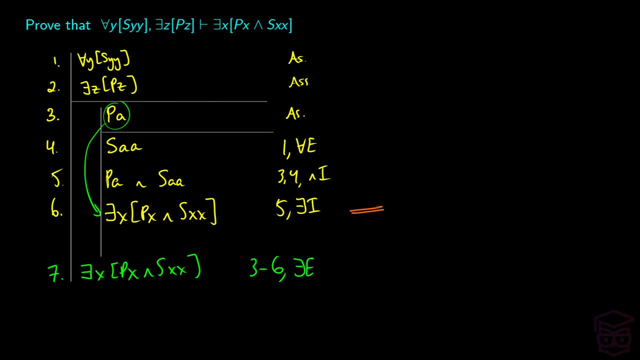 was that this step, when you do existential introduction, is a step that's often forgotten because you think in your head: we're introducing an existential, There has to be some weird requirement on it, But in actuality no, You can introduce an existential whenever you want.